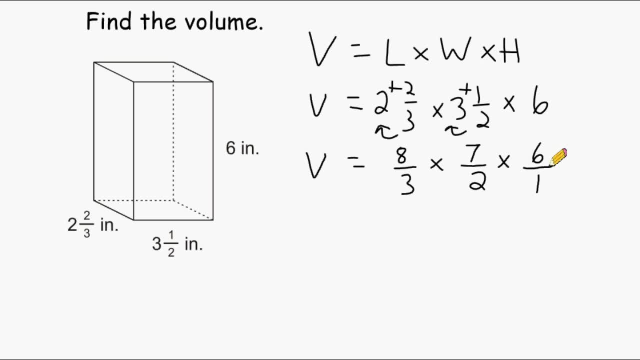 common factor. For example, 3 and 6 have a common factor of 3.. So we are going to take that common factor of 3 and divide it into each number. 3 can be divided into 3 one time. 3 can be divided into 6.. 3 can be divided into 7.. 3 can be divided into 8.. 3 can be. 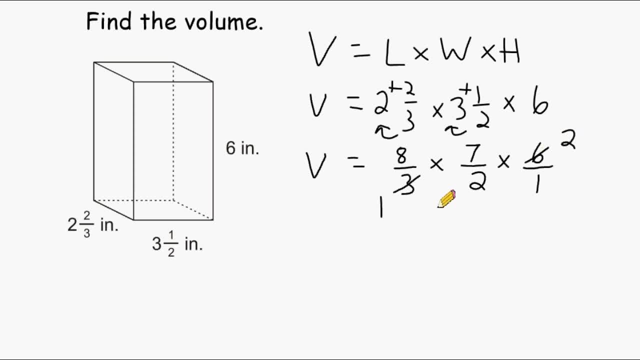 divided into 6 two times. Now we check to see if there is one more number at the top and one more number at the bottom that can be cancelled. If you have a 1, those are as small as you can reduce those, So we can ignore the 1's. But this 2 can be cancelled with. 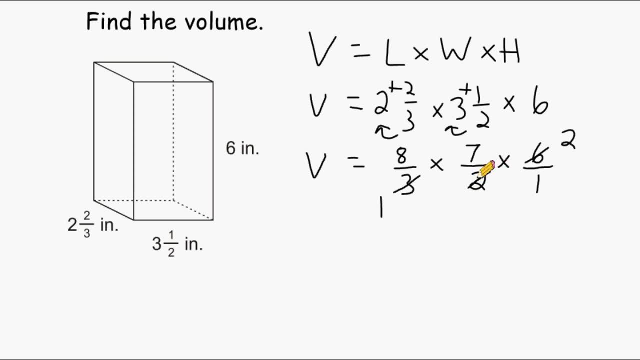 this 2 up here And if you ever have the same number on the bottom and the top, you can cancel those terms out and change those into the number 1 automatically, Because the biggest thing that can go inside itself is itself. 2 can go inside 2.. 2 can go inside 7.. 2 can. 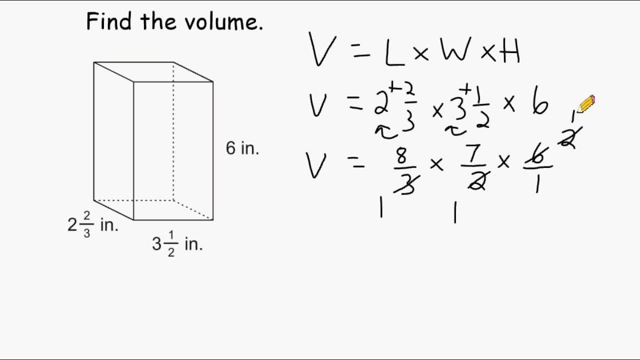 go inside 2 once And 2 can go inside 2 one time as well. So now that we have cancelled everything that's possible, we are going to multiply our remaining numerators together to get our numerator And our remaining denominators to get our 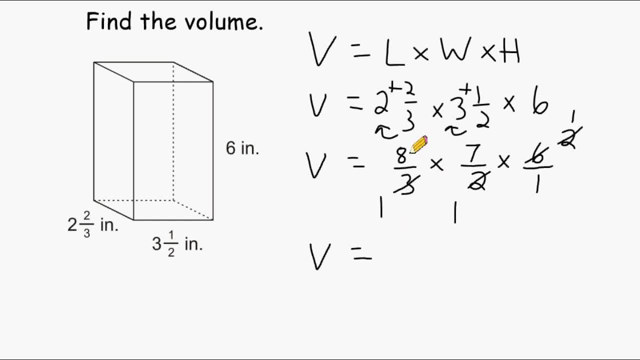 denominator. So on the top we have an 8 and a 7. So 8 times 7 is 56. And 56 times 1 is also 56. So the numerator will be 56. And for the denominator we have 1 times 1 times. 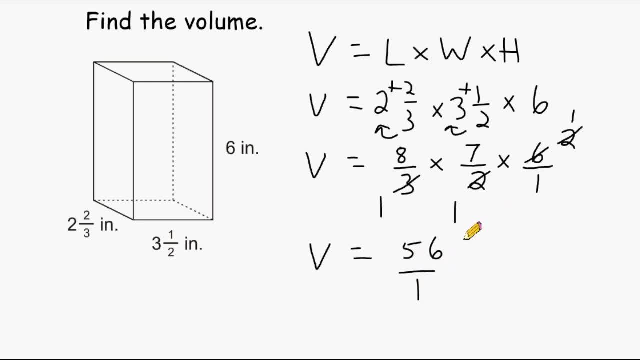 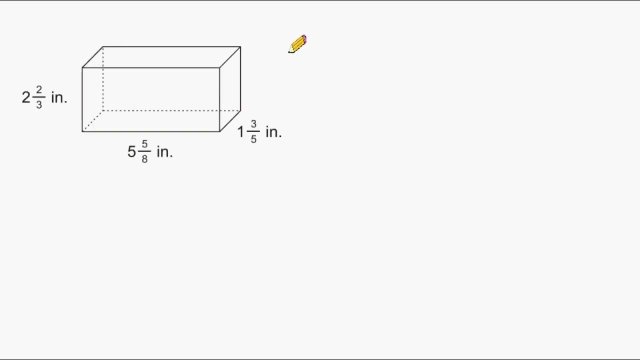 1, which is 1, and anything divided by 1 is itself. So the volume of the shown rectangular prism is 56 cubic inches. Let's try one more example. This time, instead of writing the formula, I'm going to plug the numbers into the formula right away, and I like to start with the. 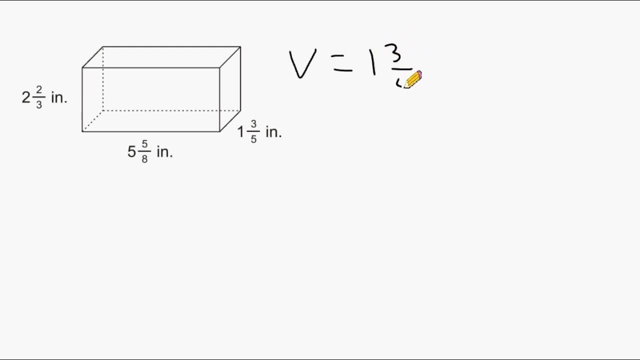 two numbers that represent the dimensions of our base. So I'm going to write one and three-fifths, first multiplied by five, and five-eighths multiplied by the height, which is two and two-thirds. Next we have to rename all of our mixed numbers as improper fractions. One and